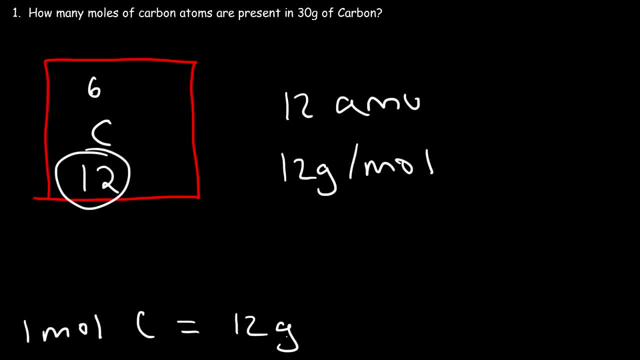 carbon atoms has a mass of 12 grams. This is your conversion factor. That's what you need in order to convert from grams to moles. So let's start with what we're given, That's 30 grams of carbon. Now, what unit should we put on the bottom here? Notice that we have grams of. 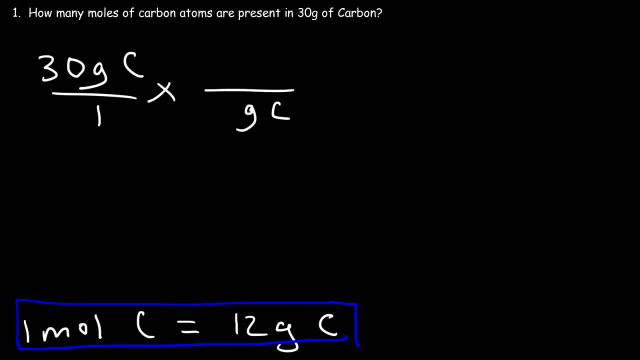 carbon on the top left. So we need grams of carbon on the bottom right, and the number that's in front of it is 12.. So for every 12 grams of carbon, there's one mole of carbon. Now you always want to set this up in such a way that the unit 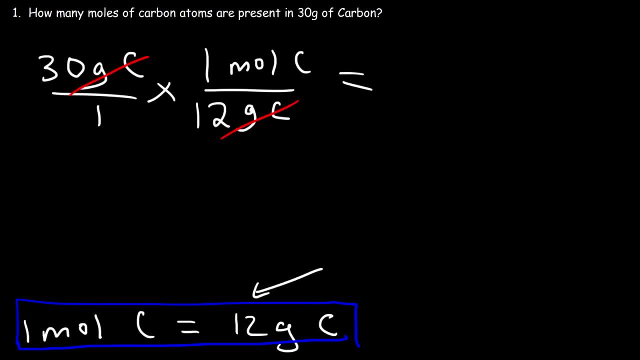 grams of carbon cancels. So here we need to divide. It's going to be 30 divided by 12, which is 2.5. So 30 grams of carbon is equivalent to 2.5 moles of carbon. That's how you can convert grams to moles. Number two: how many moles of? 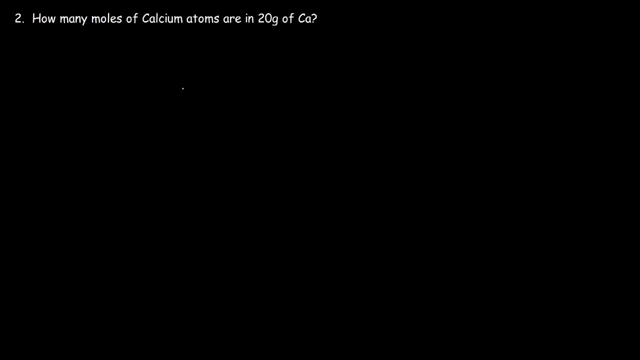 calcium atoms are in 20 grams of calcium. So first let's find the atomic mass of calcium. So if you look at the periodic table, you'll see that calcium has an atomic number of 20 and a mass number of 20.. Calcium has a mass number, or an average atomic mass, of 40.08.. So this number here, 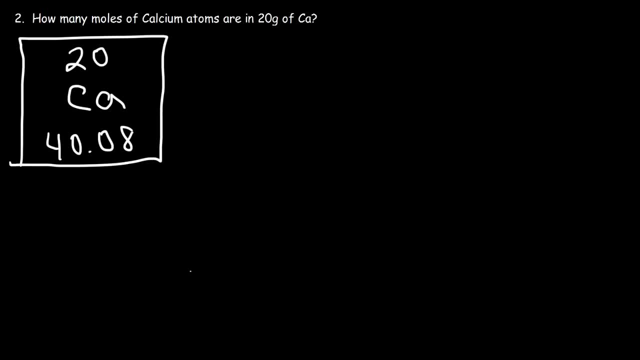 that is the molar mass of calcium, and it's 40.08 grams per mole. So what that means is that one mole of calcium has a mass of 40.08 grams. So this is our conversion factor. So now let's start with what we're given. 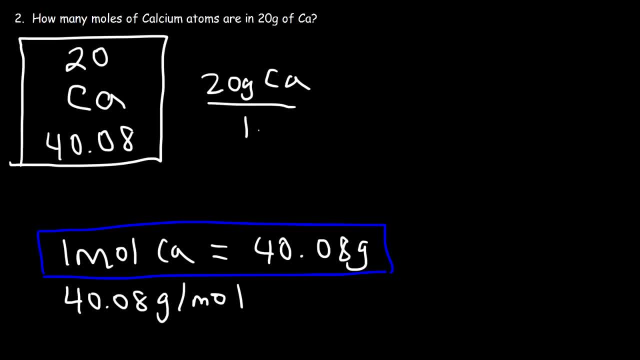 Which is 20 grams of calcium. And since we have grams of calcium on the top left, we need to put it on the bottom right. So let's put 40.08 grams of calcium on the bottom right and one mole of calcium on top, So the unit grams of calcium will. 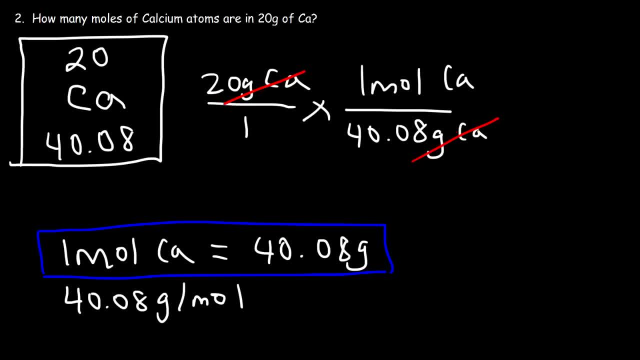 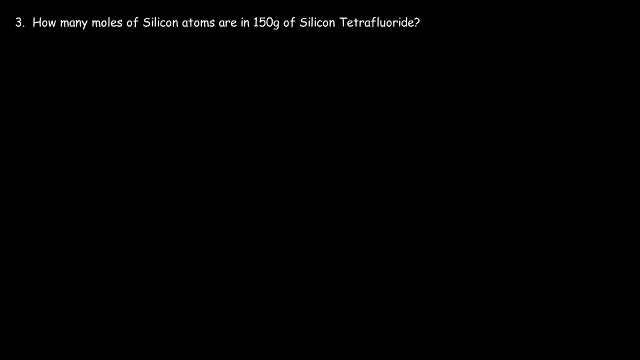 cancel. So it's going to be 20 divided by 40.08, and this is equal to 20.08.. So that's the answer for this problem. Number three: how many moles of silicon atoms are in 150 grams of silicon? 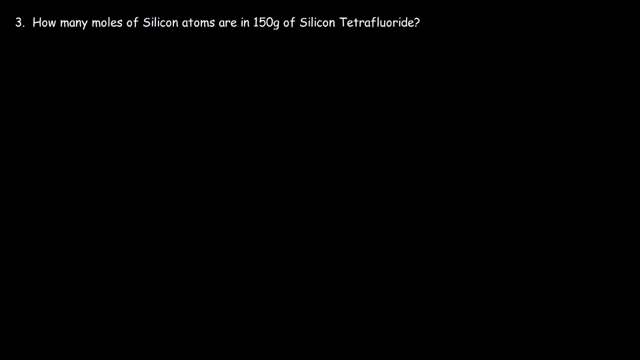 tetrafluoride. Now, this problem involves a little bit more work, So let's begin. The first thing we need to do is find the molar mass of silicon tetrafluoride. So the chemical formula is SIF4.. Tetra is associated with the number 4.. 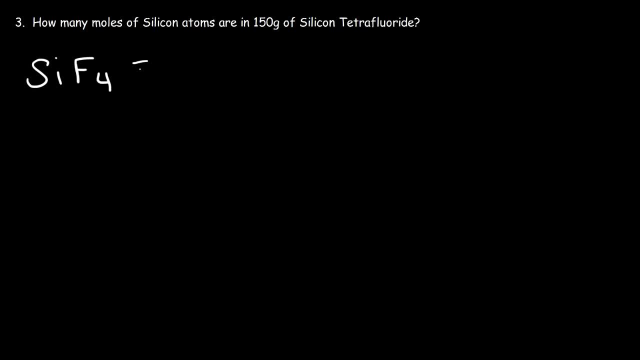 So this compound has one silicon atom and 4 fluorine atoms. According to the periodic table, the atomic mass of silicon is 28.09 and the average atomic mass of fluorine is about 19.. Four times nineteen is 76, and 76 plus 28.09 is 104.09. so that's the molar mass. so one mole of silicon. 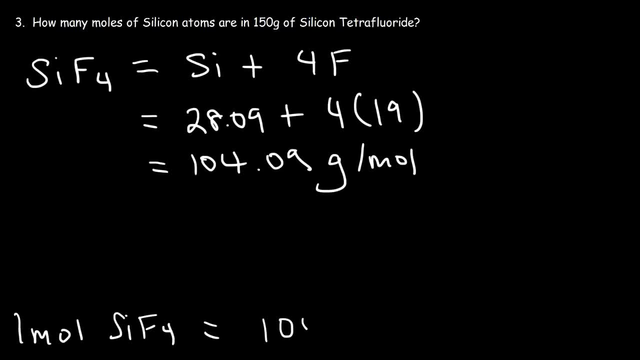 tetrafluoride has a mass of 104.09 grams. now let's start with 150 grams of silicon tetrafluoride. now we need an extra conversion step because we need to change the substance from silicon tetrafluoride to simply silicon. so that's another way in which the problem. 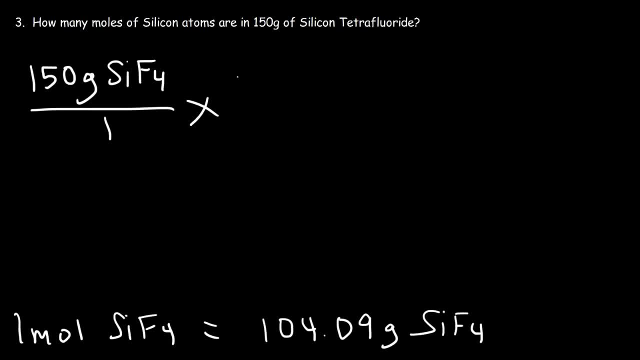 is a little bit different, but let's convert it to moles. one mole of silicon tetrafluoride has a mass of 104.09 grams. now there's one silicon atom per compound. so for every mole of silicon tetrafluoride there's one mole of silicon atoms. so the answer is not going. 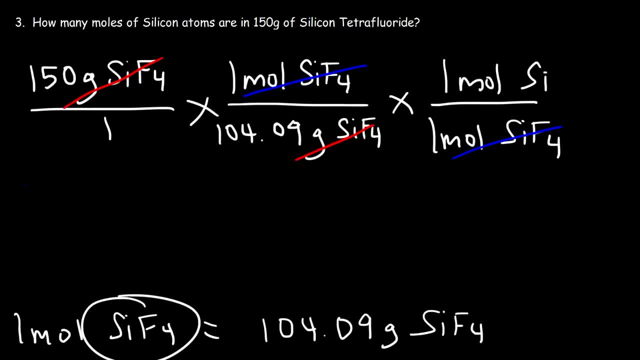 to change in this example, but for other examples it could be different. it's important for you to watch out for that step. so it's going to be 150 divided by 104.09 and the answer is 1.44 moles of silicon atoms. here's another. 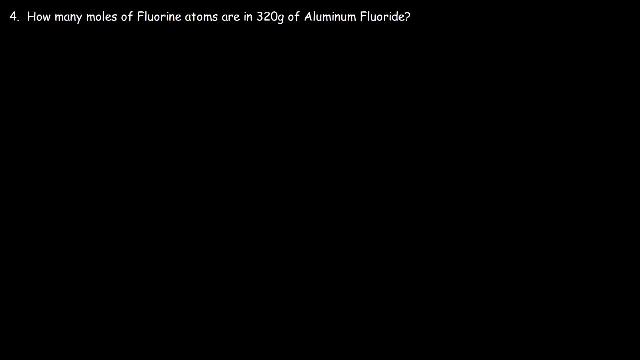 problem. that's a little bit harder than the last one. it's a few extra steps involved. how many moles of fluorine atoms are in 320 grams of aluminum fluoride? so if you want to tackle this problem, you can do that by taking the equation and find out. the actual number. 1 is 1.4-1.5-1.4-1.4-1.4-1.5-1.5-1.5-1.5-1.5-1.5-1.5-1.5-1.5-1.5-1.5-1.5-1.5-1.5-1.5-1.5-1.5-1.5-1.5-1.5-1.5-1.5-1.5-1.5-1.5-1.5-1.5-1.5-1.5-1.5.. 1.4 is 1.5 moles of silicon. so that's another way in which the 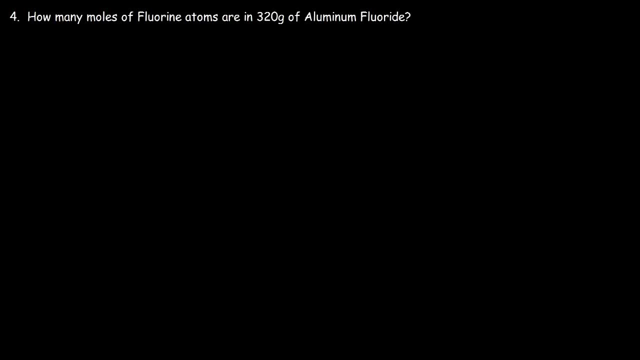 So, first, what is the chemical formula of aluminum fluoride? If you're thinking ALF, that is not the answer. What we have here is an ionic compound. The last example was a molecular compound, But for an ionic compound we need to come up with a formula. 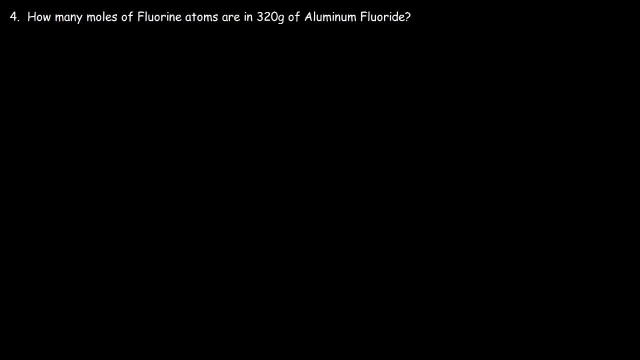 We don't have a prefix that tells us if it's difluoride or trifluoride, So we got to use the charges. Aluminum has a positive three charge. Fluoride has a minus one charge. In order for this compound to be neutralized, one aluminum ion has to be paired up with. 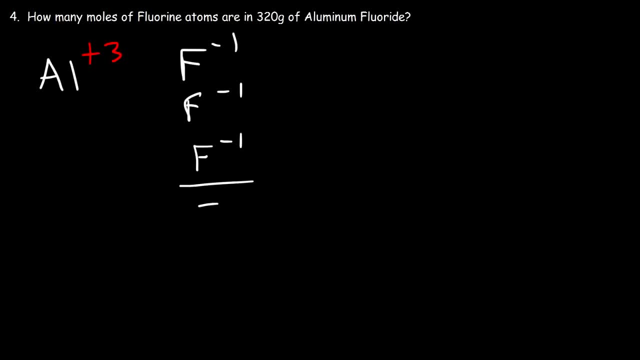 three fluoride ions So you can have charge balance. Or you could use the crisscross technique where you can exchange the charges with subscripts and just reverse them. So this is going to be Al1F3.. But if you have a liquid ion you're going to have to replace it with Al2F3.. But if you have a liquid ion, you're going to have to replace it with Al2F3.. But if you have a liquid ion, you're going to have to replace it with Al2F3.. You don't need to write chemical one as a subscript. 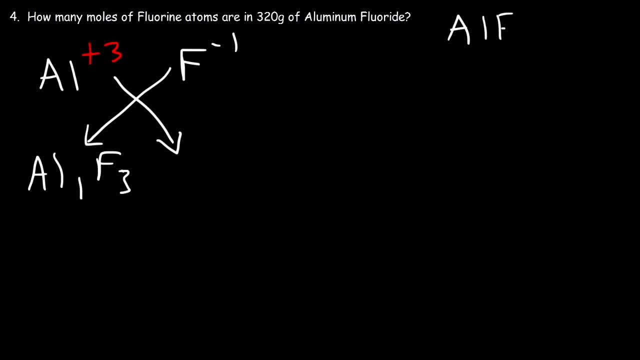 You don't need to write it. So the chemical formula for aluminum fluoride is simply AlF3.. So now that we finished that crucial step, now we could find the molar mass of AlF3.. So we have one aluminum atom and three fluorine atoms. 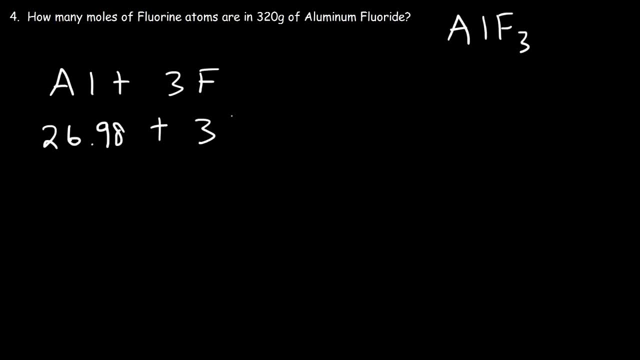 The atomic mass of aluminum is 26.98. is 19.. So 3 times 19,, that's 57, plus 26.98, that's going to give us a molar mass of 83.98 grams per mole. So what this means is that one mole of aluminum fluoride has a mass of 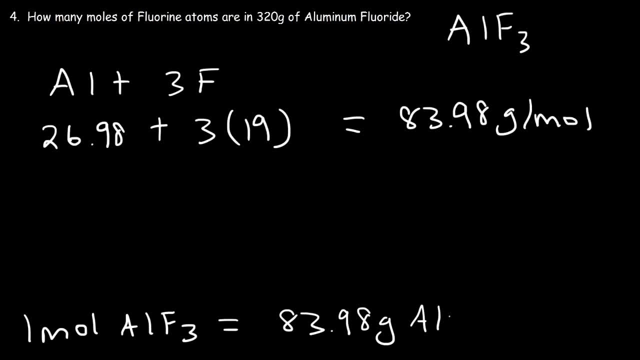 83.98 grams of Al-F3.. So now let's get rid of this And let's start with 320 grams of Al-F3.. Now let's convert it to moles. 1 mole of aluminum fluoride has a mass of 83.98 grams per mole, So that's going to give. 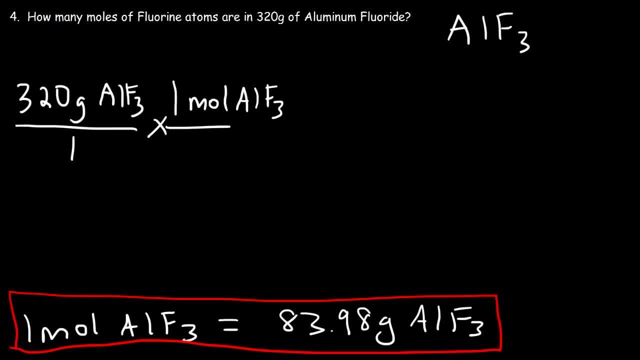 us, a mole of Al-F3 has a mass of 83.98 grams. Now we're not looking for moles of Al-F3.. We are looking for moles of fluorine atoms. So therefore we need to convert from Al-F3. 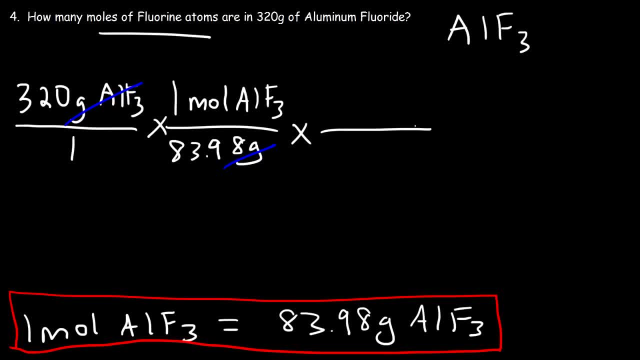 to just F. We've got to change the substance. Now notice that there are 3 atoms per formula unit. So 1 mole of Al-F3 contains 3 moles of fluorine atoms. We have a 1 to 3 ratio. So the answer is going to be 320 divided by 83.98, multiplied by 3.. So that's going to give us a final answer of 11.43 moles of fluorine atoms- Number 5.. How many moles of oxygen atoms are in 2.4 kilograms of calcium phosphate? 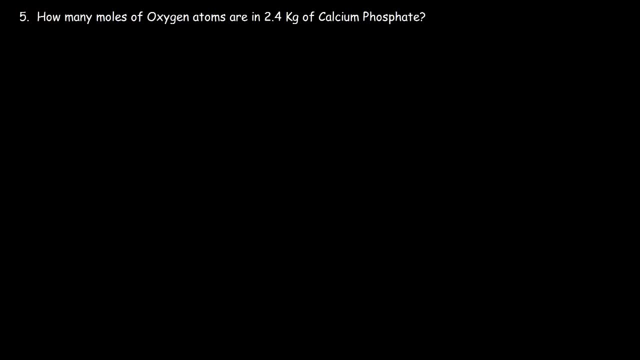 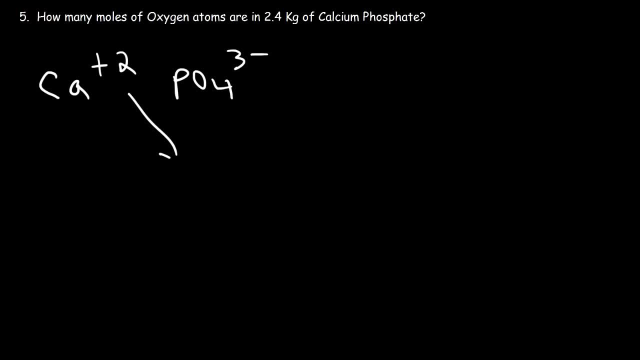 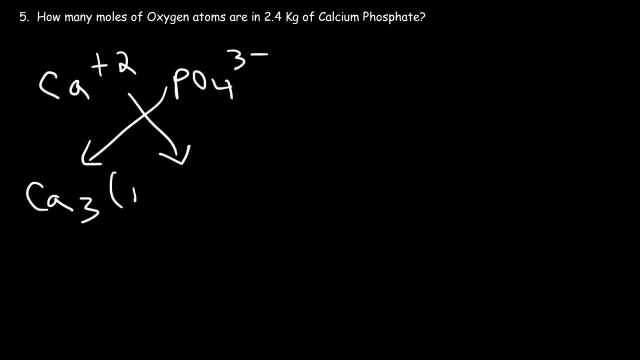 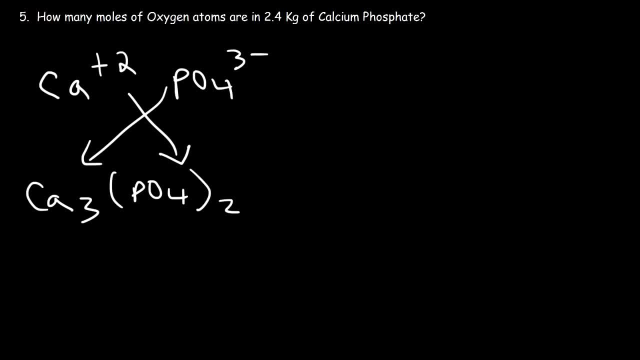 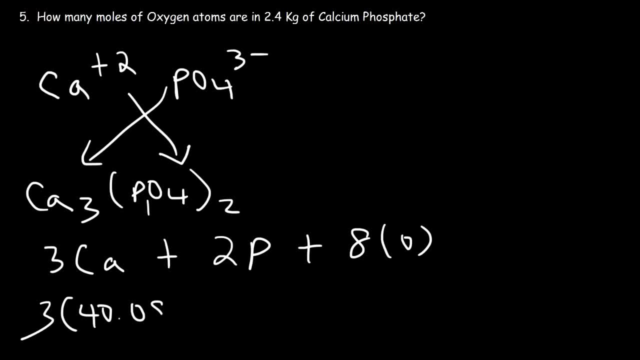 So the molar mass of calcium, that's 40.08.. The molar mass of phosphorus is 30.97.. And the molar mass of oxygen is 16.. So you can type this in exactly the way you see it in your calculator. 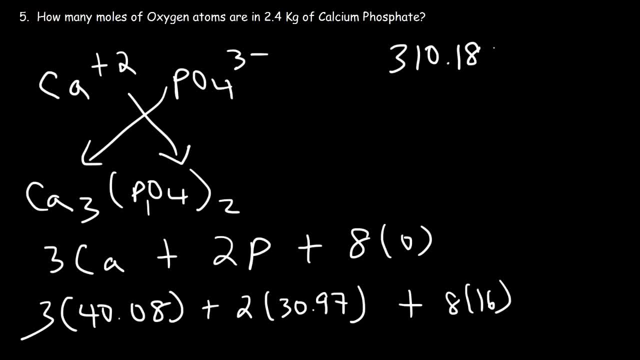 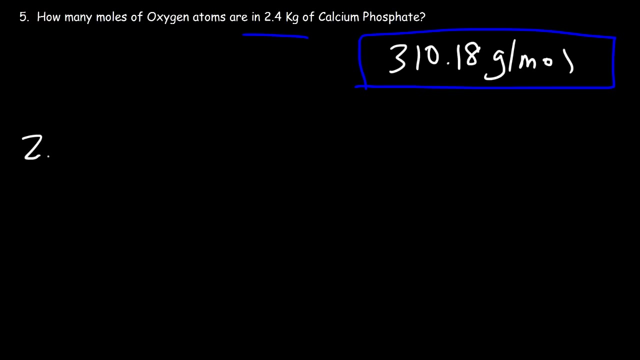 And you should get a molar mass of 310.18 grams per mole. So now we can finish the remainder of the problem. So let's start with what we're given, which is 2.4 kilograms. Now, before we can convert this to moles, we need to convert kilograms to grams. 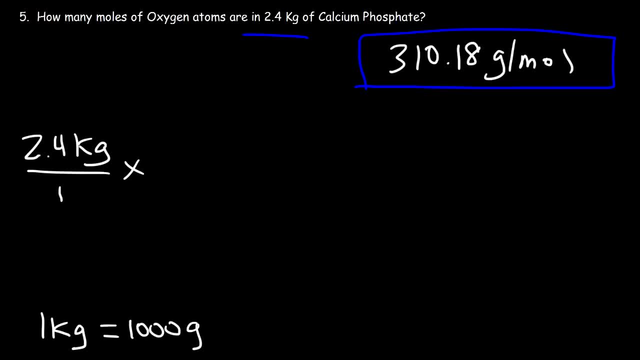 1 kilogram is equal to 1,000 grams. So let's put 1 kilogram on the bottom and 1,000 grams on top. We want the unit of kilograms to cancel. Now let's convert grams to moles. 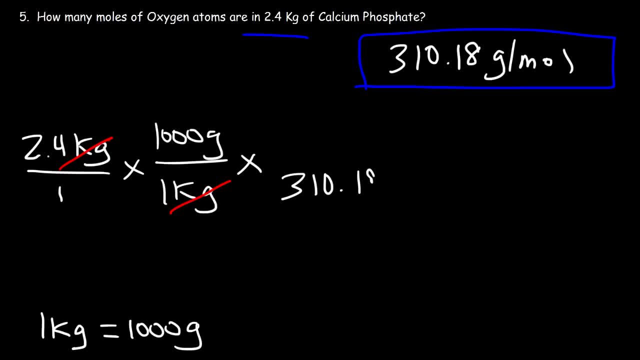 There's 310.18 grams of calcium phosphate per 1 mole of Ca3PO4.. That looks like a 9.. Now our goal is not to find the moles of calcium phosphate, but rather to find the moles of oxygen atoms. 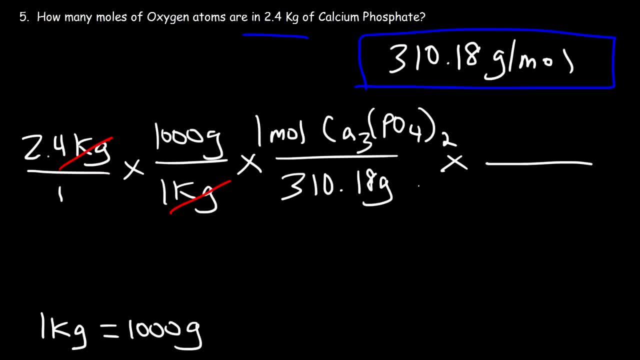 Now notice that there are 8 oxygen atoms per formula unit. So we can say that 1 mole of calcium phosphate contains 8 moles of oxygen atoms. So now the unit grams cancel and the unit moles of calcium phosphate will cancel as well. 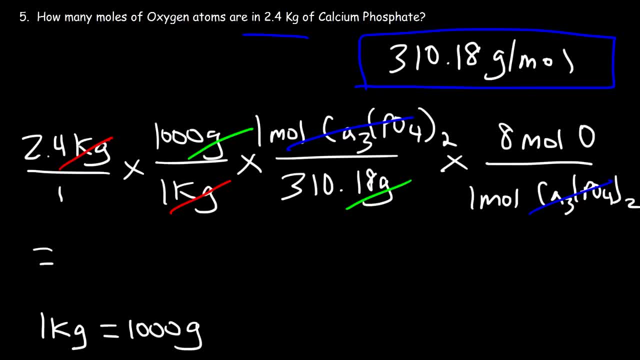 So it's 2.4 times 1,000, which is 2,400, divided by 310.18.. That gives us 7.737, and then multiply that by 8.. So there are 61.9 moles of oxygen atoms in 2.4 kilograms of calcium phosphate.